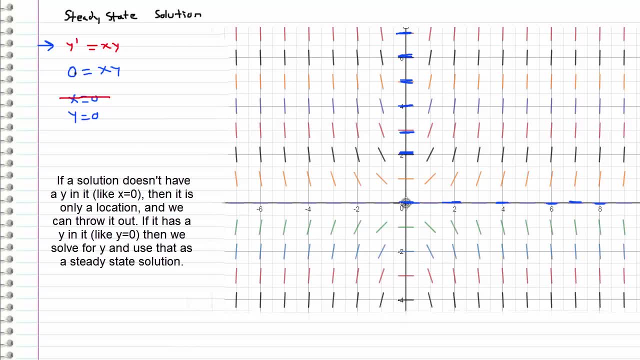 location. We're interested in an actual function that gives us a steady state solution, which is: y is equal to zero, which means that all across this, all across the x axis, the slope is zero And this represents our steady state solution, because the slope is not changing. But now we can look at stability, And this is part of the reason why we drew a slope field, because we can easily categorize the steady state solution by looking at stability. We see that if we were 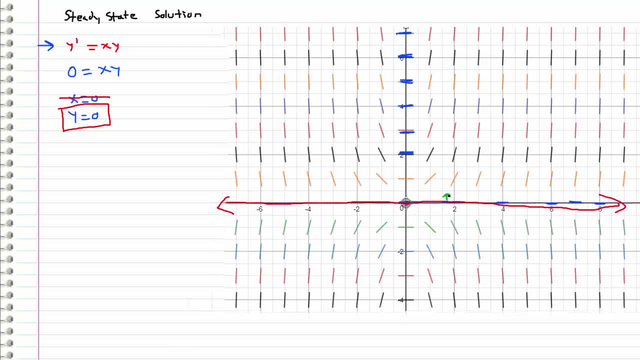 were to deviate just a little bit above in this direction that our solution would go and diverge this way, because we have to follow the slope lines. And similarly, if we were to deviate a little bit below the x-axis, our solution would deviate and diverge completely down here to. 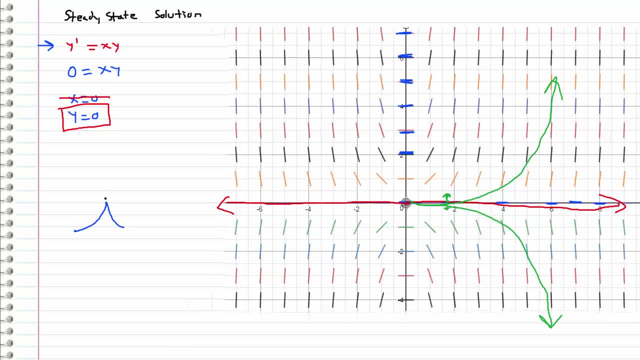 negative infinity. So this is kind of like a ball balancing on this little corner And if it were to tilt just a little bit it would roll down here, And if it were to tilt a little bit other way, it would roll all the way down there. It would never come back And we could say that. 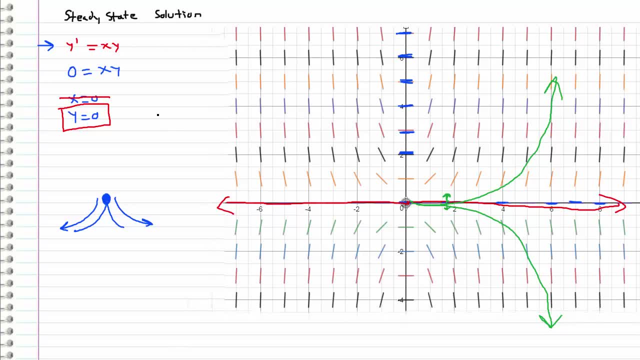 this ball is unstable. So this steady state solution right here, this y equals zero. because of the nature of the slope field and because that little deviations caused the solution to diverge to infinity, we characterize this as unstable. So anyway, that's true. 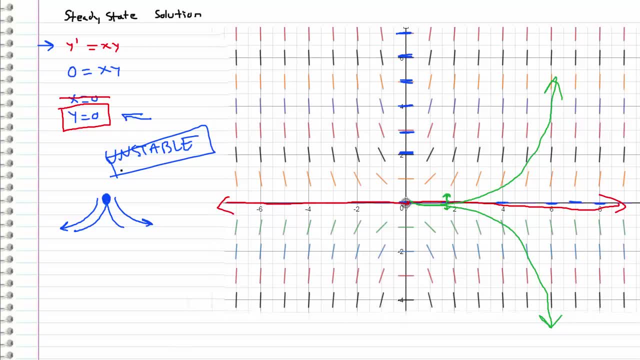 That's just a quick little example. Thanks for watching, And I'll see you guys in the next video, where we will talk about classification of first order differential equations And then after that we will start solving them.